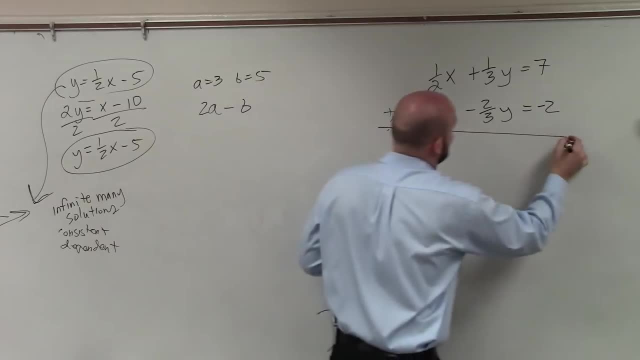 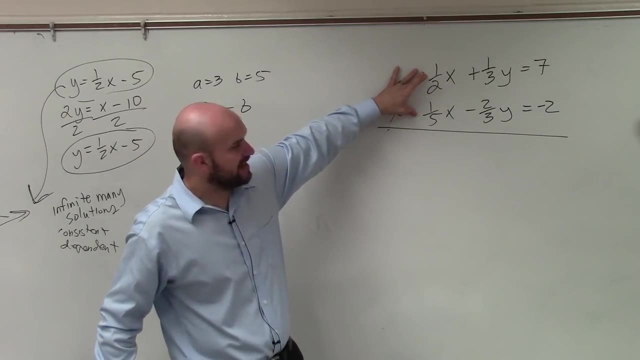 is just adding or subtracting our two equations. And if we add or subtract these two equations, we want to be able to get a coefficient of zero. So if I add or subtract one-half x- plus or minus negative, or one-fifth x, am I going to get zero. x Does one-half plus one-fifth. 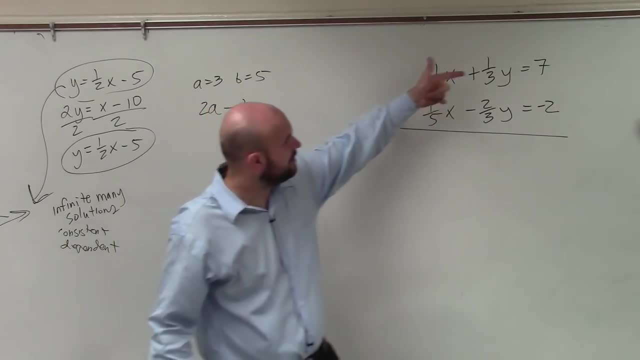 give you zero. Does one-half minus one-fifth give you zero? No, What about one-thirds and two-thirds? Is one-third plus one negative two-thirds going to give you zero? No, So they're not going to give us zero. 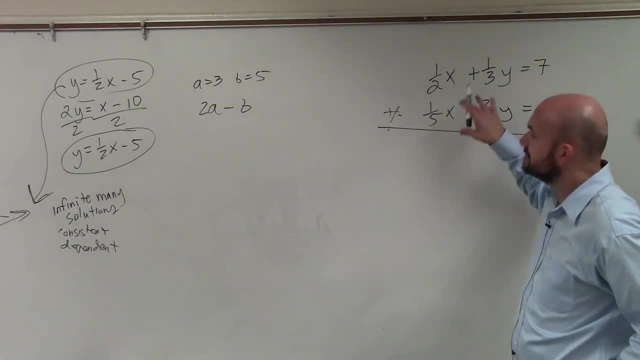 So the next thing that I'd recommend to do is get rid of your fractions. So to get rid of my fractions I want to get rid of. the reason why these are decimals is because two does not evenly go into one, So you want to multiply it, so you want to get the numerator. 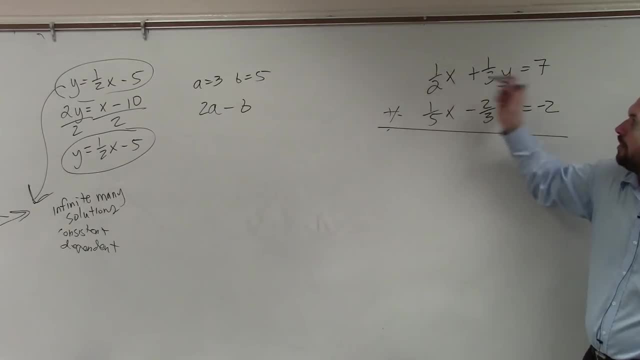 into a number that is evenly divisible by two. Well, you also need to get into a number that is evenly divisible by three. So what is the smallest number? that two and three are Six, Six. So I'm going to multiply everything by six. Now, same thing over here. We need 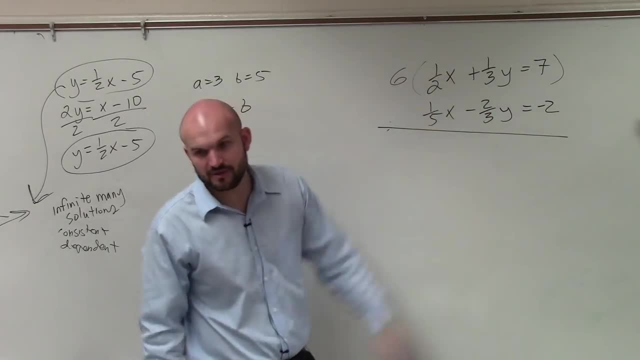 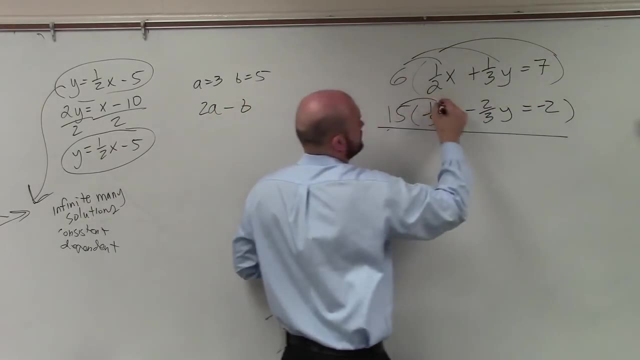 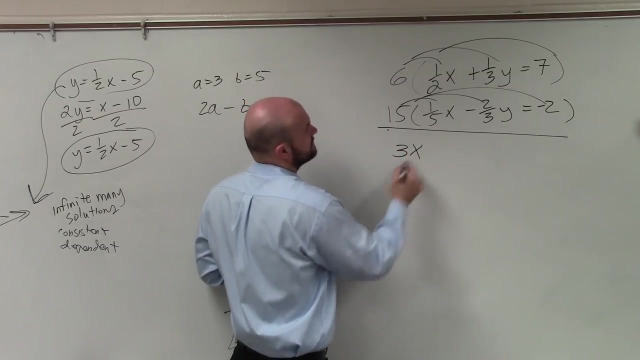 to find a number that five is divisible in two and three is divisible in two And that smallest number is. Then we apply the steward of property. Do you have to do all three? Yep, you have to do all three. So, six times one-half, x is going to be three x Six times. 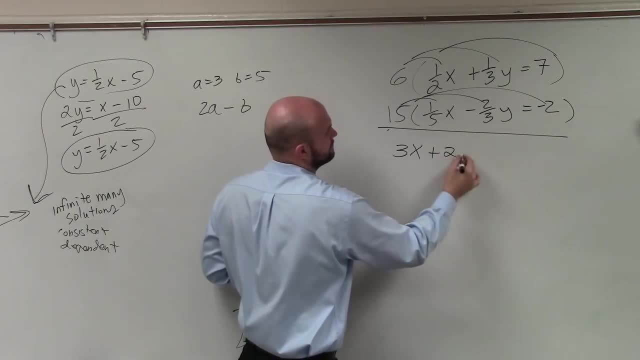 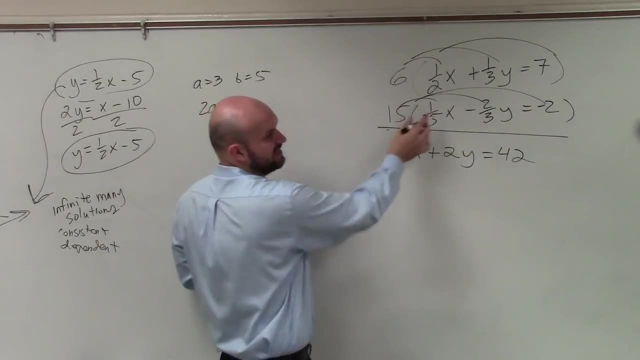 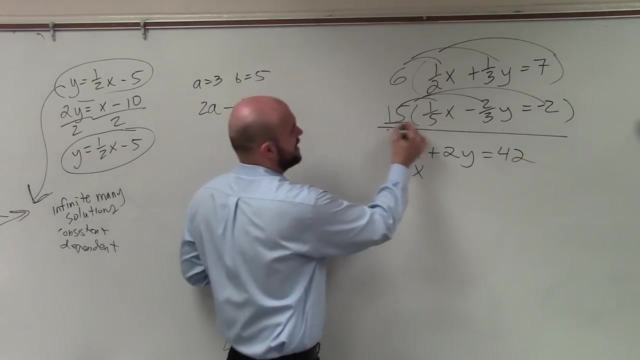 one-third y is going to be two y Six times seven is equal to 42.. Follow me Then I do this: one Fifteen times one-fifth x is going to be three x Fifteen times negative two-thirds. just multiply over Fifteen times. 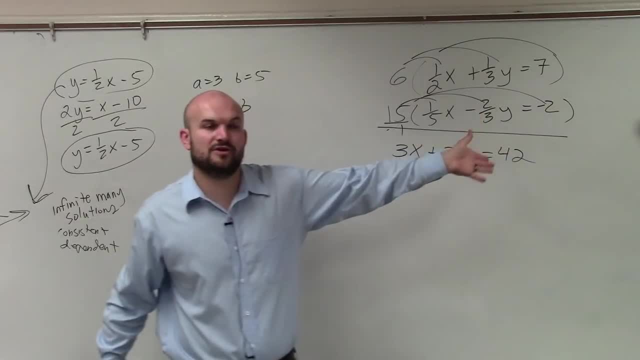 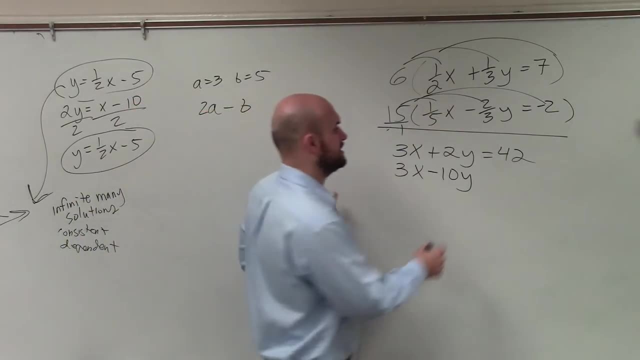 negative two is negative 30.. One times three is three, so negative 30 divided by three is negative 10.. Follow me, You want me to show that. Okay, Fifteen times negative two is equal to negative 30. Now, 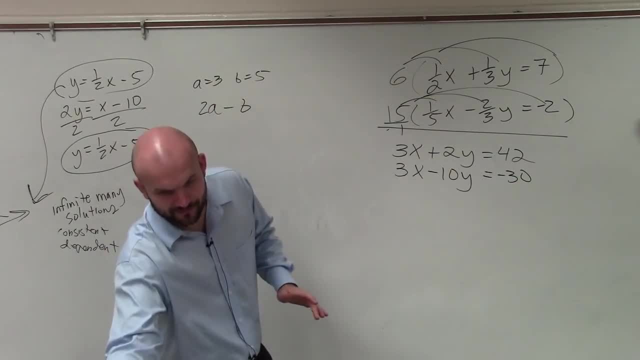 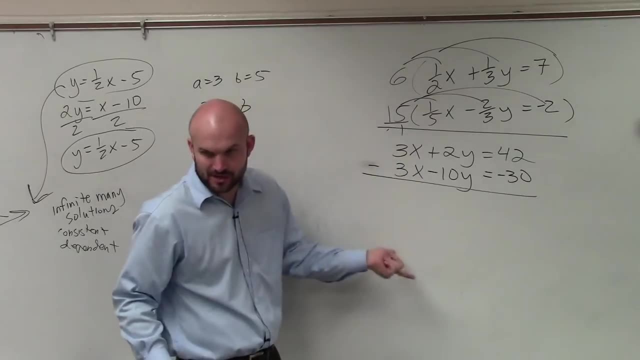 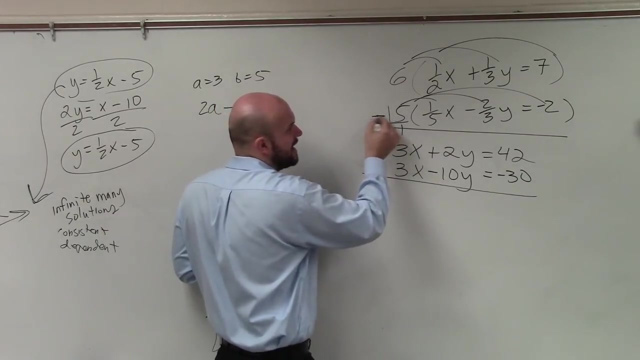 You can see now, not if I add them, but if I subtract these two equations. now I have them: zero right, Which is cool. However, I don't really like subtracting. I don't think you are. you would too. So, rather than multiplying by fifteen, what would happen if we multiplied?